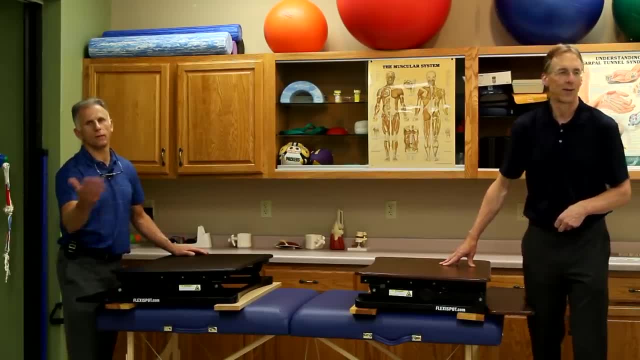 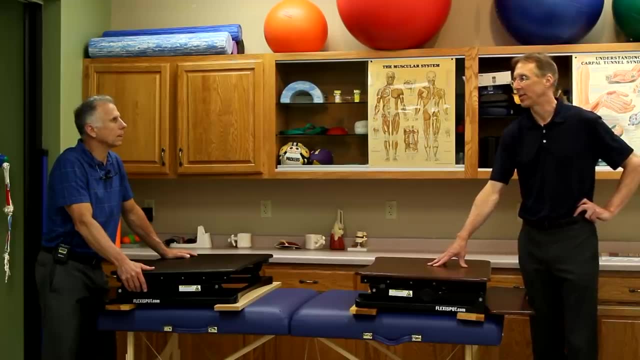 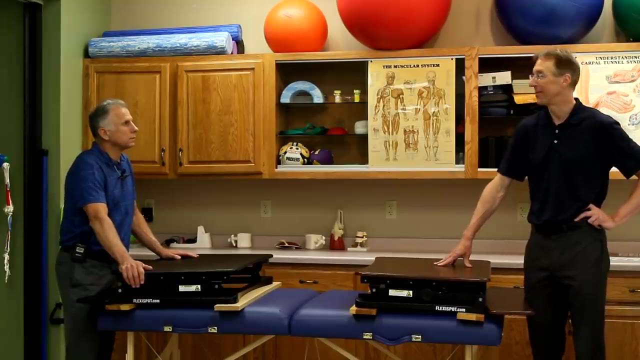 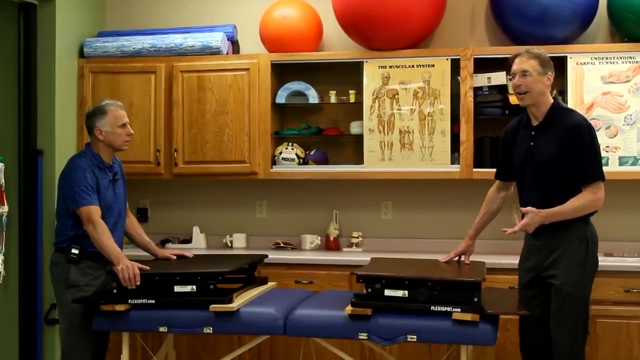 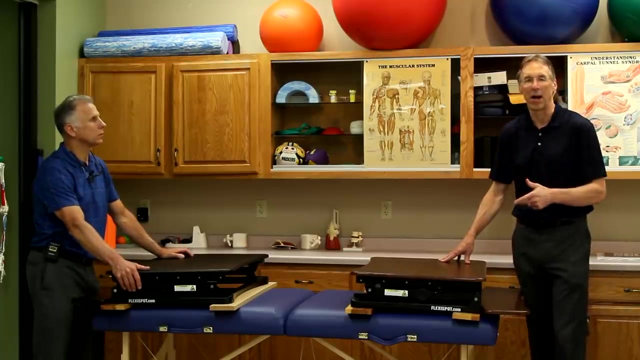 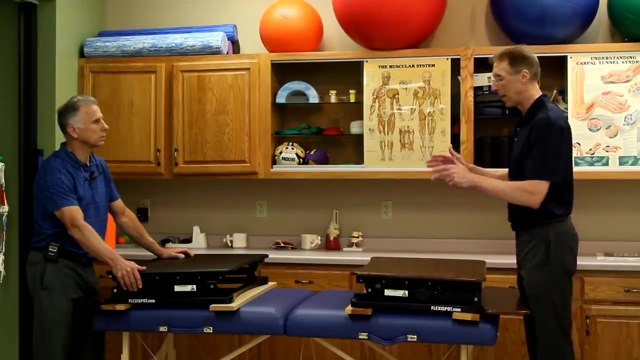 Did I say cause? No, I just wanted to re, you know, make sure we were, you know, Alright. so you know it's funny. we got this. you know, we got one of these desks- probably what? almost a year and a half ago, Yeah, I would say so. And the first time I got the desk and I didn't use it, I was like it was too much work for me to convert everything around. Sure, We did another video on it and I'm like God I got to listen to ourselves what I'm saying here. This, you know, this really is not good for you because there's going to be some more reasons I'm going to give you a little bit later on, Sure, Of why you want to stand up. So I went ahead and made the change and I really liked it. I I actually what I did is I had my computer, I got two computer screens and I had two. 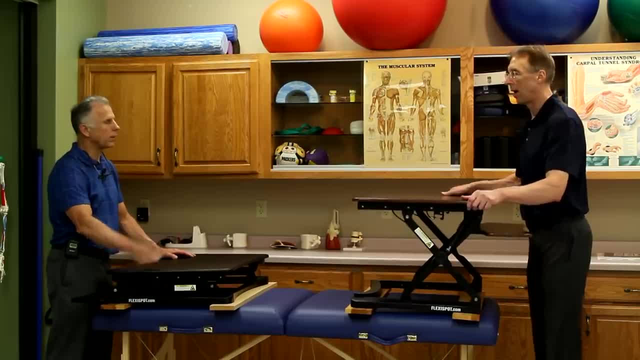 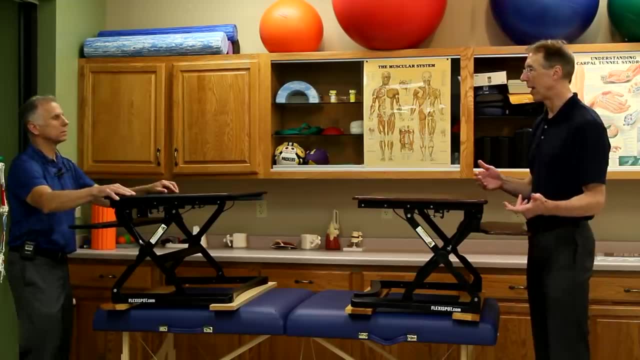 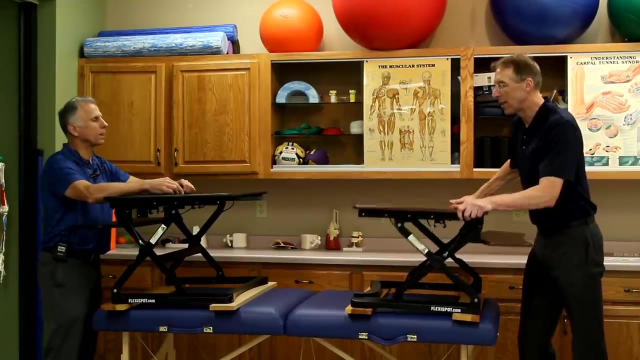 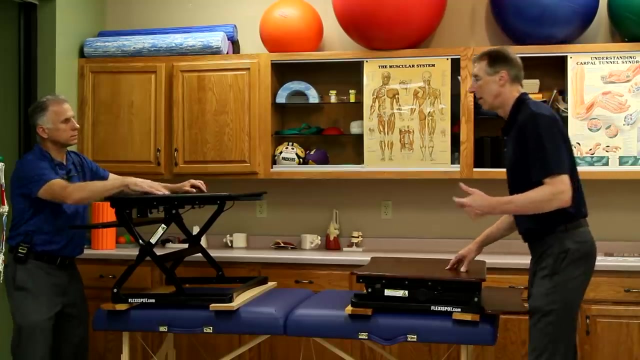 of them. Sure, I have one that I keep kind of in the raised up position, Boy, that goes up nice, Yeah, it goes up nice. and one hand, and I have one in the lower position for the seated one. Sure, And I found out that I I hardly ever even use the seated one. now I, I stay standing most of the time. You feel comfortable, I feel comfortable Standing, yep. So these are the things, the changes that I noticed, that happened to me. The number one change that happened to me is I used to get pain right. show me, yeah, do you got a? a? Where where is my stick, Bob? Yeah, there you go Here. 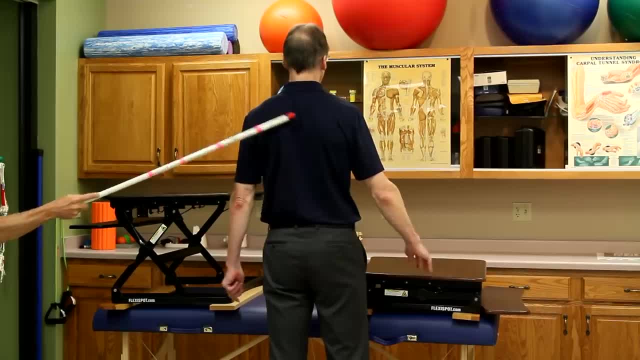 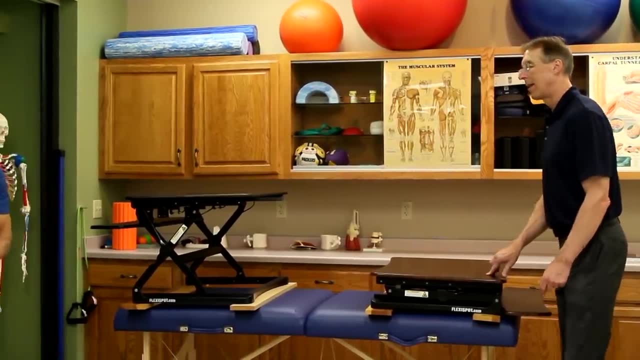 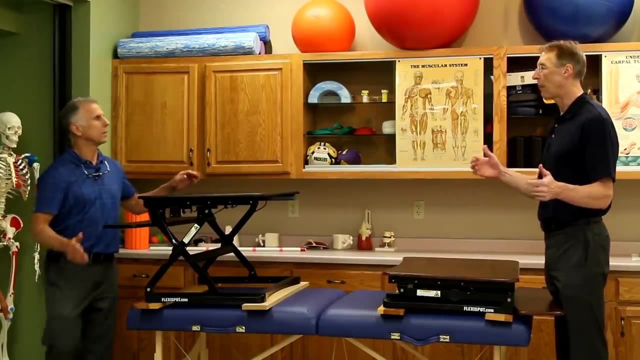 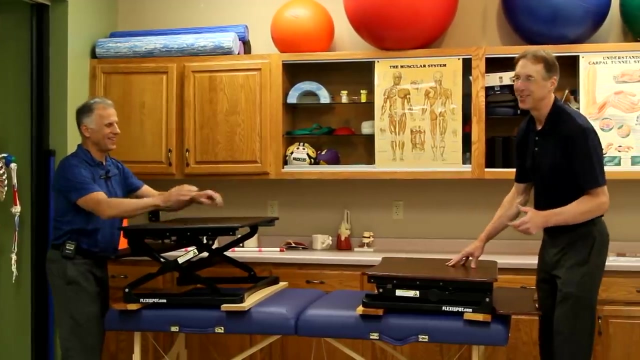 Here. Oh yeah, it's pain right. Yeah, Just kidding, Right in that area here, right between the shoulder blades- Very common. it's typically from poor posture that you're not aware of because you're working on the computer. I'm on the computer, I'm as aware of posture as anybody and I do posture exercises every day. Yep, And my wife would walk by and go: you got bad posture, you got bad posture. So you know as she likes to do. I hope she doesn't watch this video. I love you honey. Yeah, I hope she doesn't watch this video, But it just seems like no matter what, gravity wins. 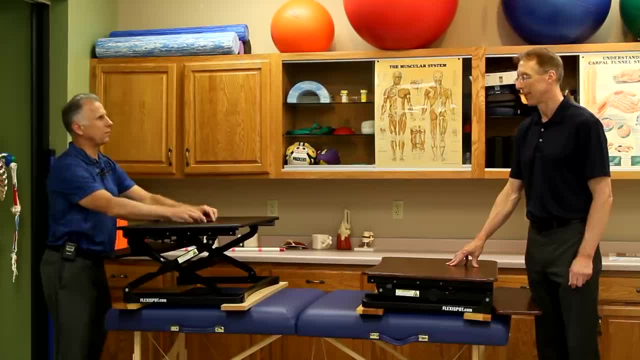 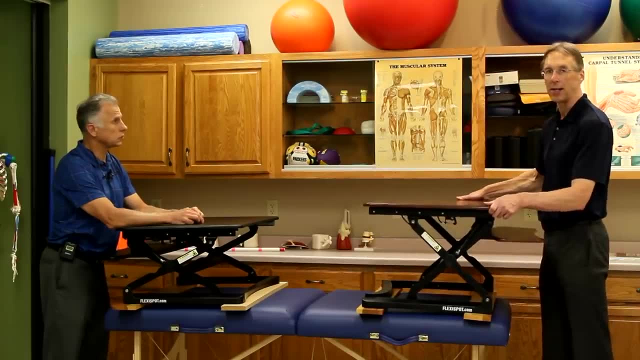 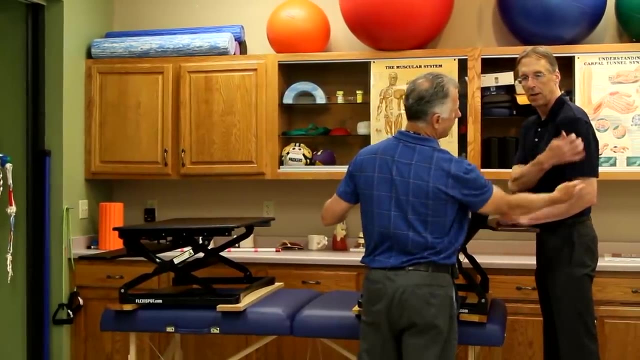 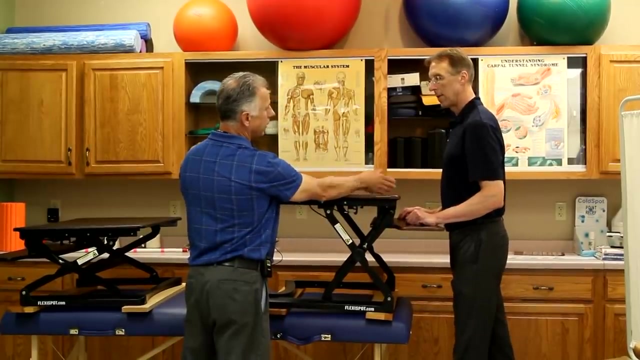 out on these things, doesn't it, Brad? Well, especially when you're focused on something else, Yeah, you get focused on a task. So I started doing this and you know, I started bringing this up, and I'm six foot six, by the way, and this thing fits me really nice actually. Look at that, This hits me right. perfect, Do you see this, Brad? Yeah, if we're looking at the angle of his elbow, Yeah, you want this vertical and you want this horizontal, or a little bit less than horizontal. So it's got the lower key tray. If the key tray was up here, that would be too high. I had to raise up the screen, though I had to put some books underneath it to raise up my screen. So I'm going to put some books underneath it to raise up my screen. So I'm going to put some books underneath it to raise up my screen. So I'm going to put some books underneath it to raise up my screen. So 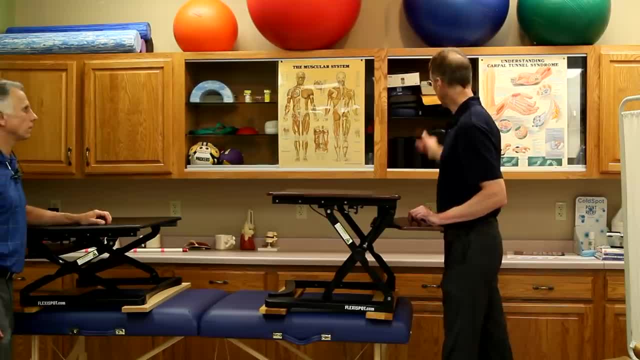 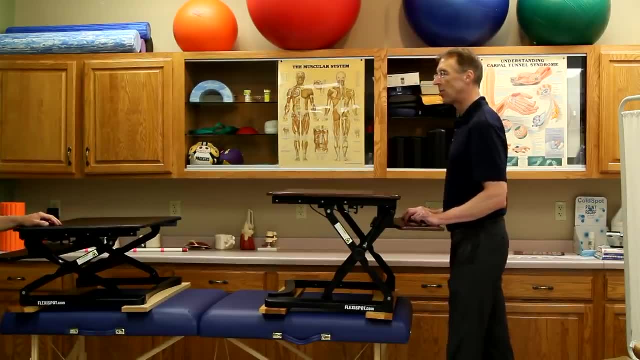 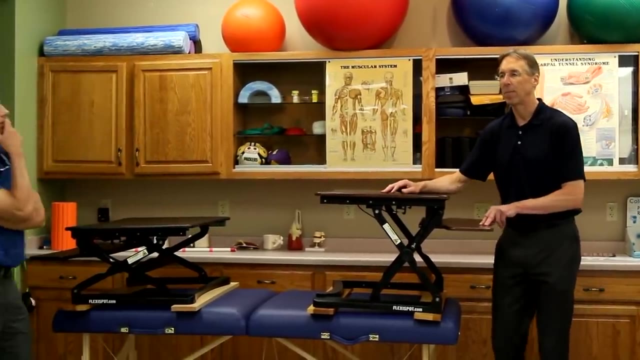 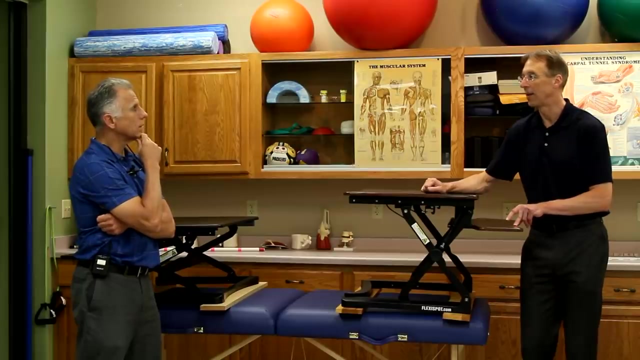 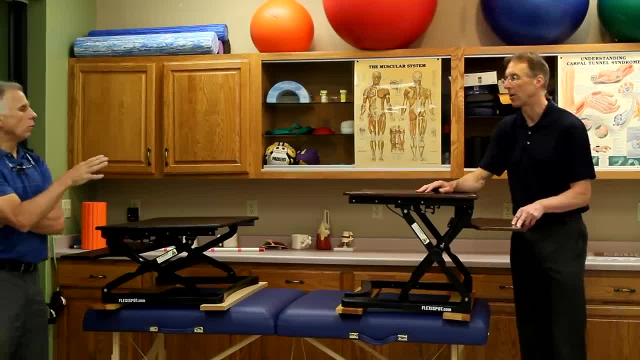 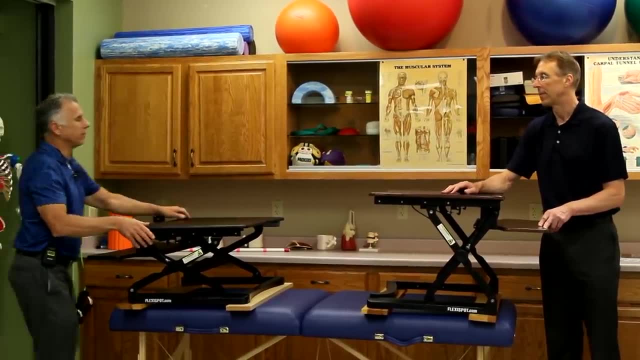 Convinced him to do so, So he's gonna make the change and see how it works out. One point I do want to make is if you're wondering it's like I'm not gonna stand all day at work, Well, you don't need to, and that's the idea of the variability. You can stand for 20 minutes. 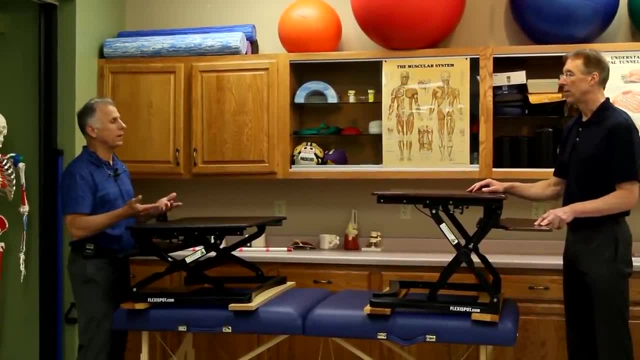 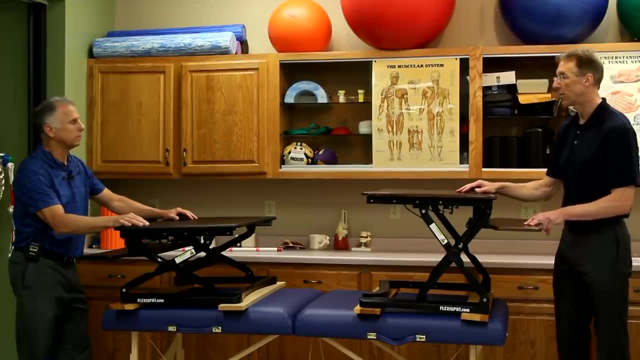 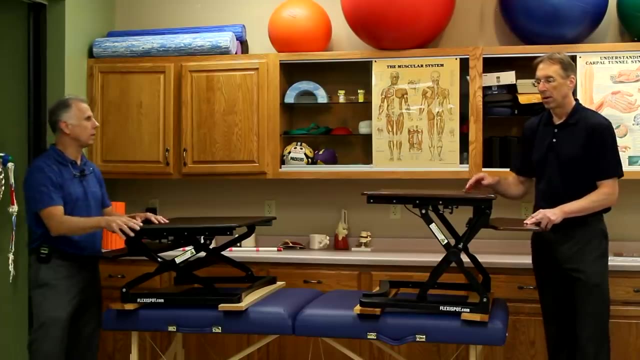 Sit for five minutes. There's a ratio that they recommend, actually, but it's actually 20 minutes standing, Eight minutes sitting and then two minutes moving. So they're recommending some exercise. We'll show a couple you can do: or go walking, Go to the filing cabinet, go down the hallway, whatever. 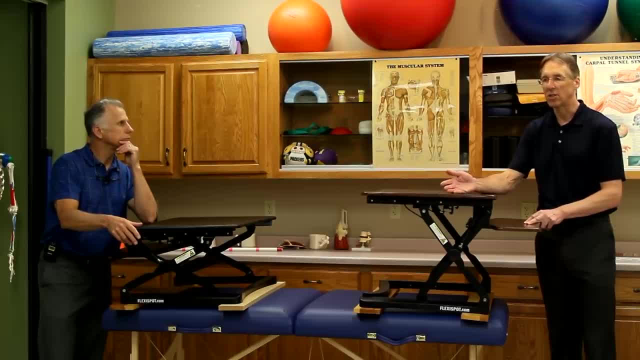 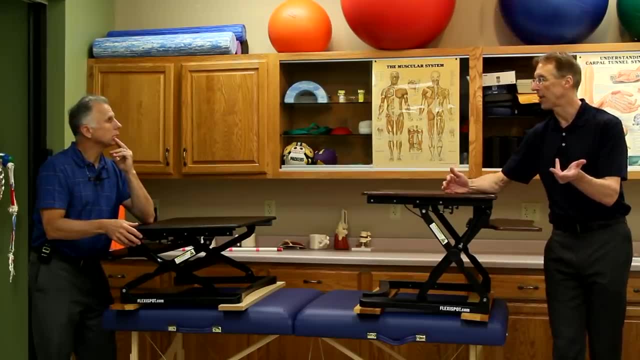 Now, if you're gonna get one of these, make sure you hit the link below. We're gonna at least get you 5% off, and yeah, we get a small fee from this too, Which I'm gonna be upfront about it, but we use it to help offset the cost of making these videos. 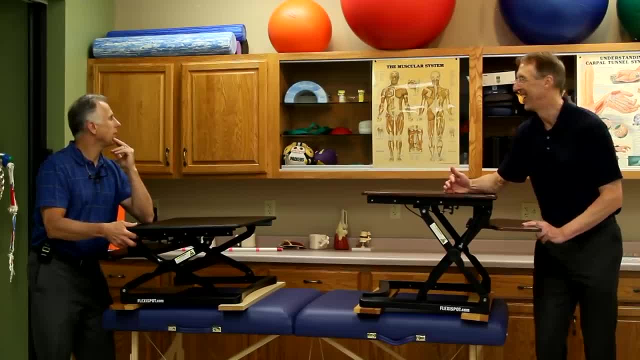 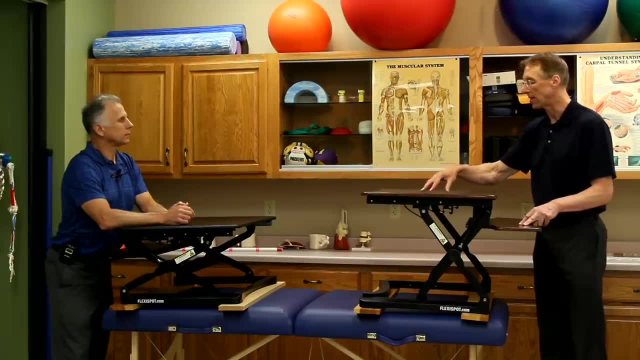 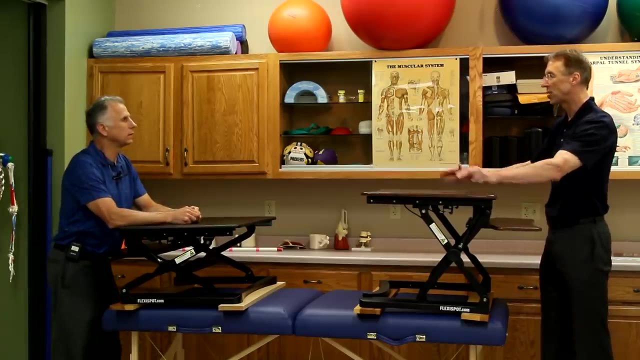 Which I'm sure you can see a very high production. Well, yeah, we've got to get some money to crack the crooked. Everybody's complaining about it, but these are really fine desks. The thing is, these have been tested 6,000 times, Brad. They took it up and down 6,000 times, Yeah, and it's 35 inches good size screen. 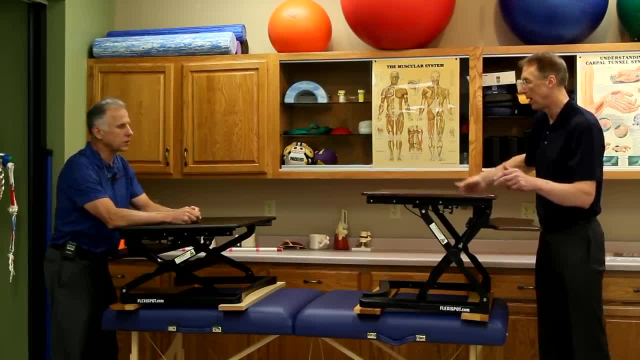 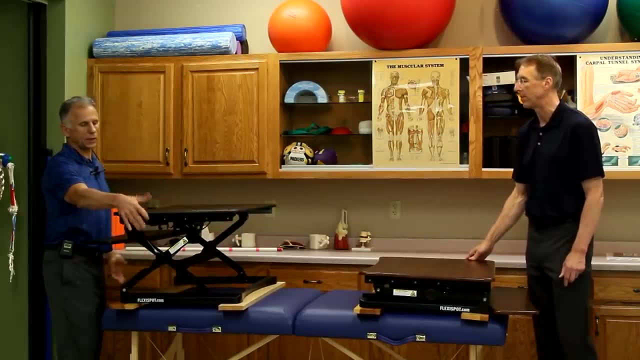 It's heavy-duty, It holds a fair amount, It's a commercial grade desk And it's a one-handed thing. here You can just do it with one hand. I mean you gotta push with both, but I mean it's one hand that brings it up and down. There's just one lock on it. 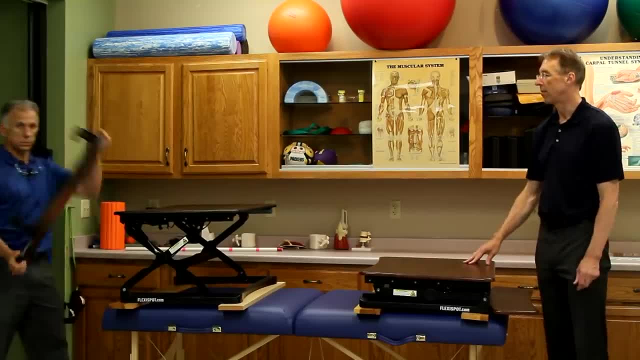 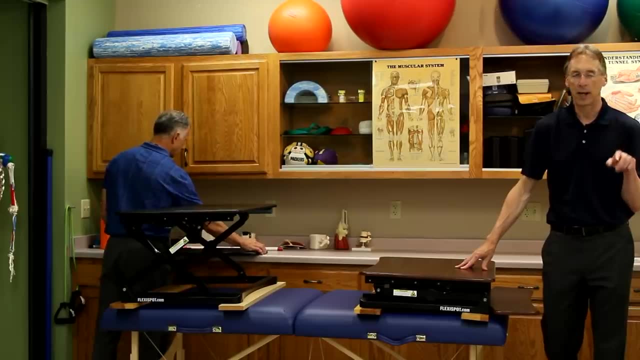 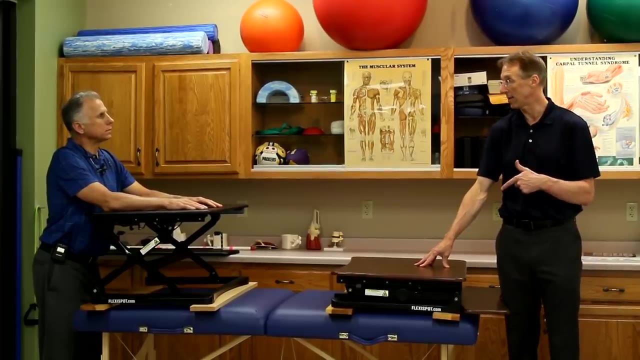 And this tray does remove really quite easy. Very nice. So again, hit the link below. The other thing I want to mention: there was some additional benefits, Brad, I was going to mention that You can get from this. there's a decreased incidence of heart disease with people who stand more.